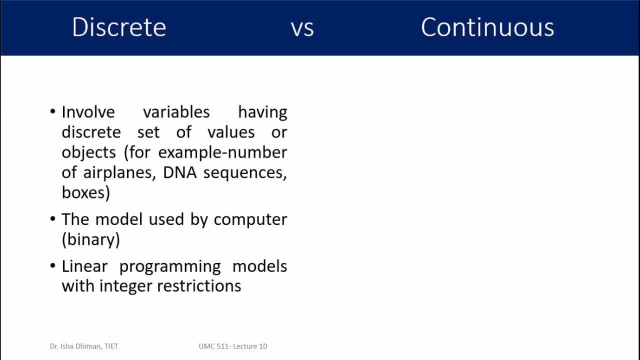 are counting the number of something, how many number of hours is required, how many number of persons are required to complete the job, or how many boxes or so, something which can be counted in a discrete manner. So that means your underlying fundamental variable is a discrete variable. So that kind of model is a discrete. 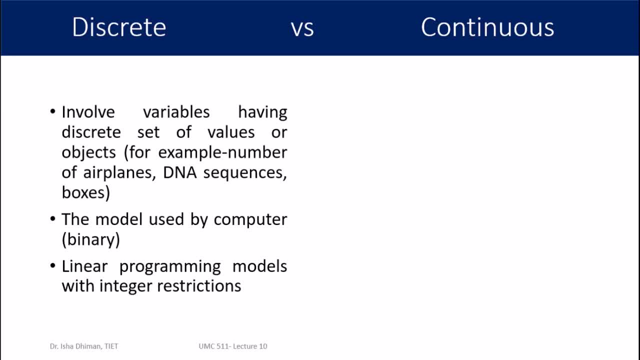 mathematical model, For example the model used by computer. So whatever language or whatever commands you are giving to your computer, it is taking it in the form of binary information that either it is one or zero for it. So that's one way to understand that the model used. 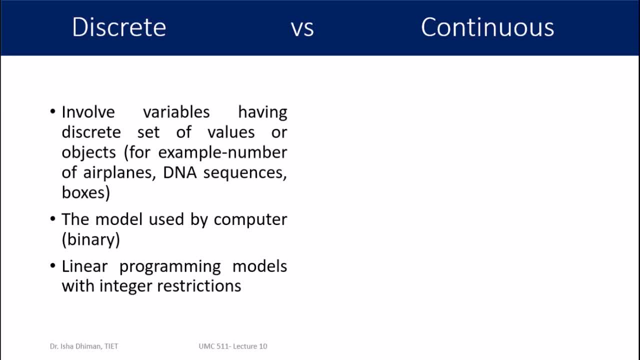 by algorithms or the computers. internal processing is a binary model and it's a discrete model. Another example which you can well understood because recently you have- you might have studied this course: linear programming, in which, if we have the integer restrictions on the variables that suppose the variables. 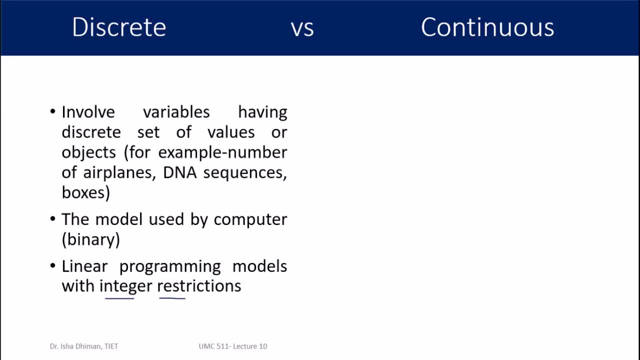 are denoting the number of persons or the number of units to be transported from one particular source to a destination. so since this is number of something, so that number is going to have integer values: it can be 20, it can be 10, it can be 15, or it cannot have a continuous range. 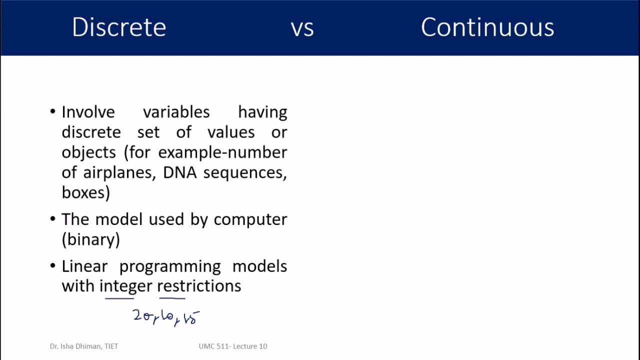 of values. these kind of models are called discrete models. discrete models can further be actually divided in two categories: one is known as semi-discrete and another is known as fully discrete. although right now I'm not going to go into detail of these two further categories, this will really depend upon whenever we are studying a particular model, then if 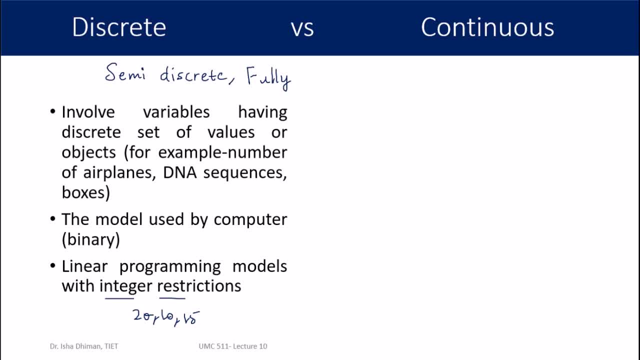 there I will feel the need. okay, we need to discuss the fully discrete version of it. then I'll definitely take it up, but otherwise these words should be clear in your mind: that semi-discrete or fully discrete is a category of discrete model. so for the time being, you can understand. 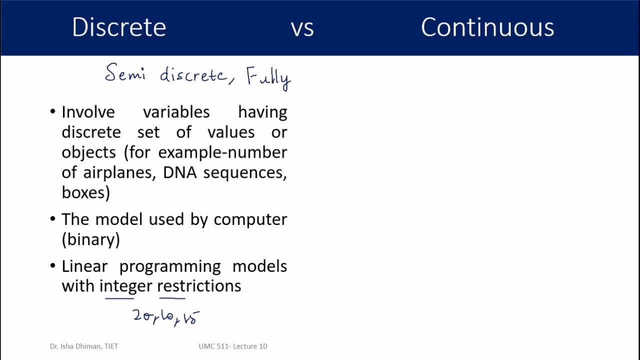 semi-discrete means one of the say, some of the variables are discrete while others are not, and in fully discrete models every variable is a not continuous or a discrete variable. on the other hand, for continuous variable, we have obviously it's now understood that these involve variables having continuous set of values. so usually these models are: 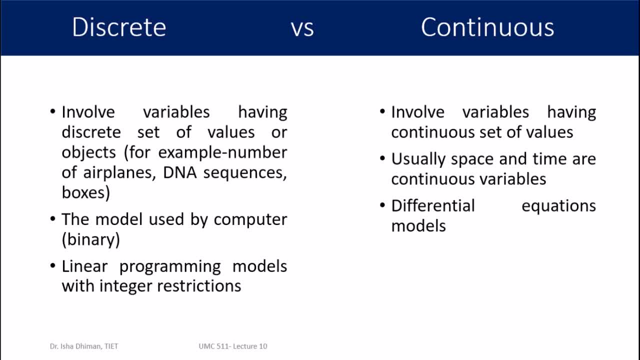 those models which contain space and time, because space and time are continuous variables, so these models are generally framed in terms of these variables. so space can be one dimensional, two dimensional, three dimensional as well, or whatever be the dimension of it, but it's always treated as a continuous space. 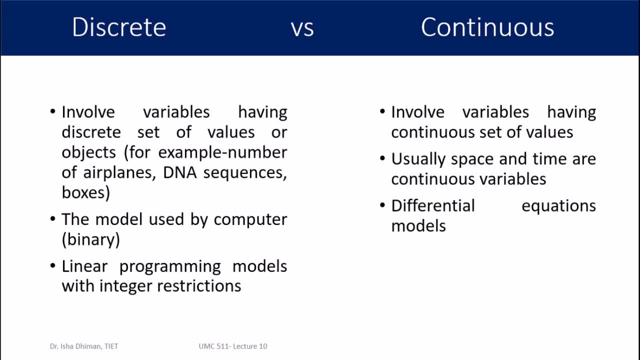 the example is differential equation models and recently in this course we have studied the population growth models in which we were looking at the population of something. you can say the one is definitely a discrete number, but it was varying with respect to time. so time is something, a continuous quantity. so whenever you represent anything with the differential, 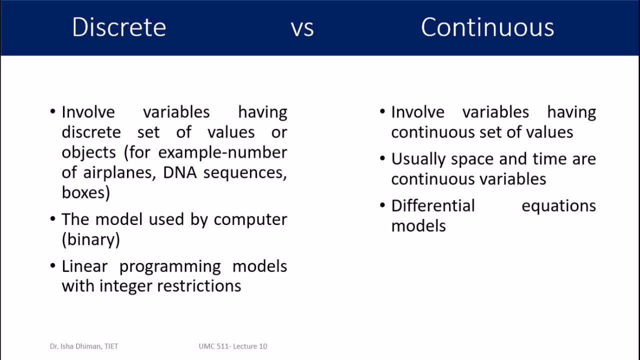 equation. so that's precisely a continuous mathematical model, because you have to assume the continuity of the variable. only then you can differentiate it. so most of the models which are formulated in terms of differential equations, they are nothing but the continuous kind of models. so we can talk about these in more detail when. 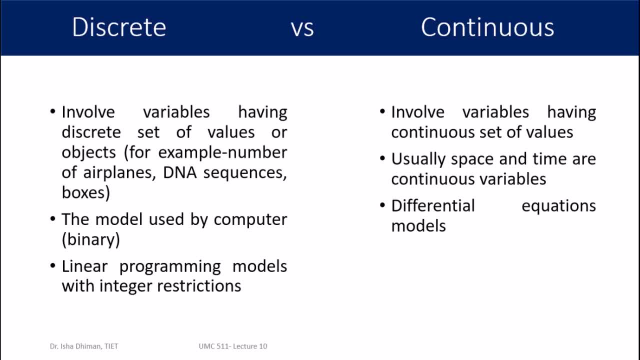 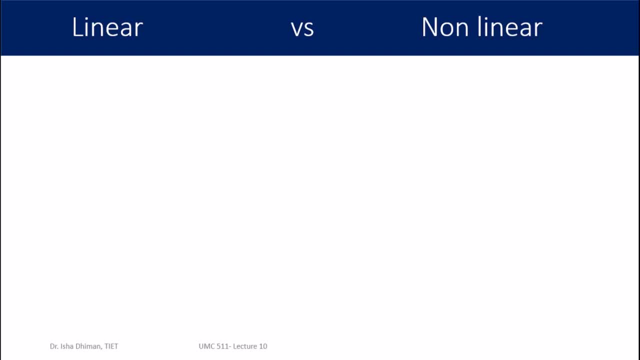 we come to the next lecture, be studying the specific models. so now let's take the next class: linear versus nonlinear. in our earlier classes, most of us are already familiar with these terms. what do we mean by linear and what do we mean by nonlinear? although in terms of the mathematical models also there 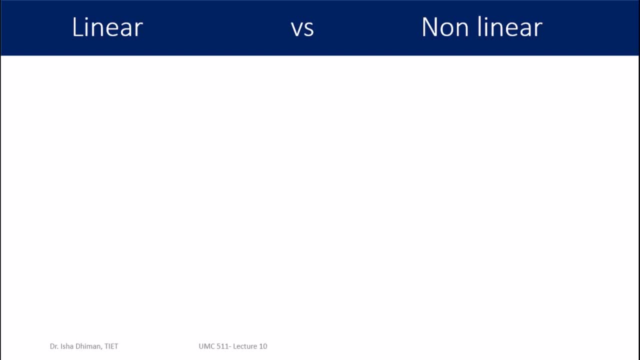 is no precise distinction, there is no line of identification which clearly distinguishes linear versus nonlinear. but I have tried myself, tried best from myself, that whatever best definition I can give you for that, okay, so this is the precise way we can understand linearity. if all the operators in a mathematical model exhibit linearity, then the resulting 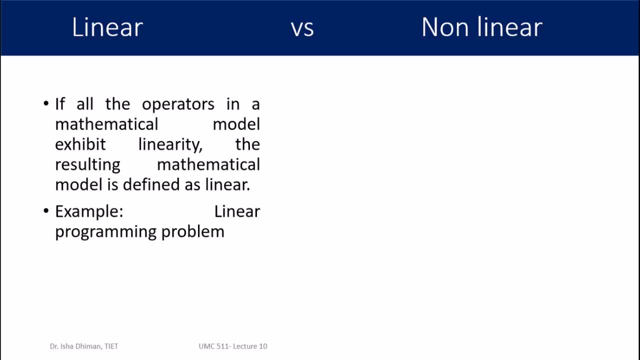 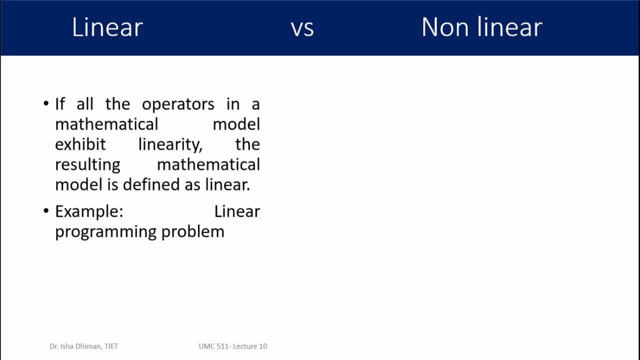 3y plus 4z. it cannot be x into y, into z. it cannot be x square or y cube. so we know what do we mean by linear kind of expressions. so those models are called linear models. example again, linear programming problem, because in that every expression is a linear expression of the 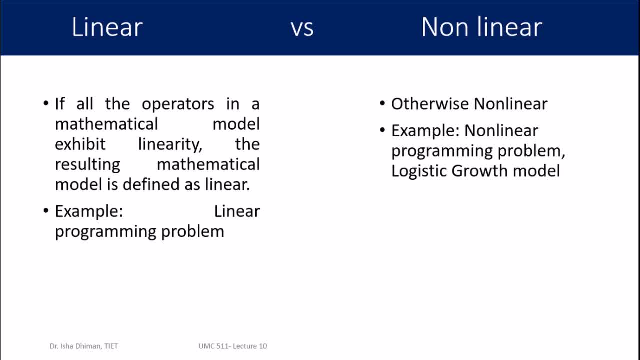 variables on the other side. nonlinear models are those models which obviously, in which linearity is disturbed, for example, two variables are multiplied with themselves, x into y. kind of factors are occurring there. some square is coming, some other function is coming, so the nonlinearity is there. exponential function is coming, logarithmic functions are. 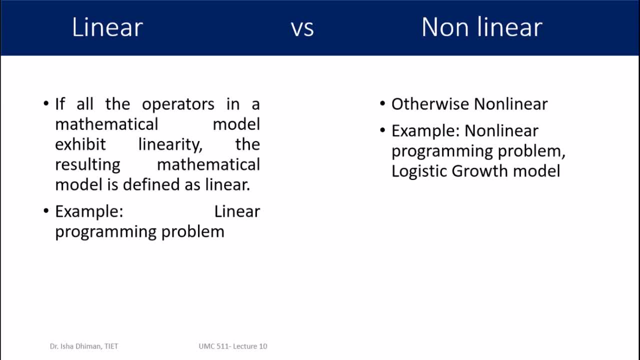 present there. so that gives the nonlinearity in the model example is a nonlinear programming problem. and if you talk about in the recently discussed population growth models, then we know that the logistic growth model is a nonlinear model because the fundamental base upon which that model was derived was this: we wanted to see the effect of incorporating 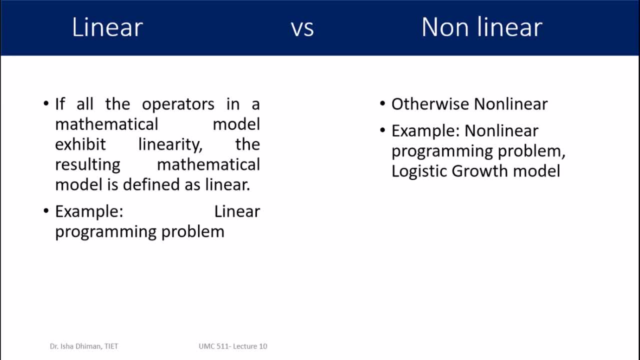 nonlinearity in population growth model which made it appear better than the other linear model versions of the same. so logistic growth model was also a nonlinear model and again I would say that this is not the precise way you will find these definitions in books, because it really depends upon the context of the model, that how. 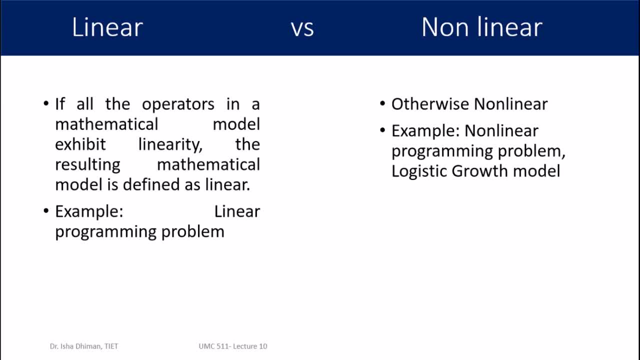 we are going to tackle with the linearity and nonlinearity. so, again, I will leave this to the specific problems, when we will be discussing that. whether to categorize that model as linear or nonlinear, that definition can also vary depending on what problem we are modeling. but this is the general idea. now lets take the third category: static vs. 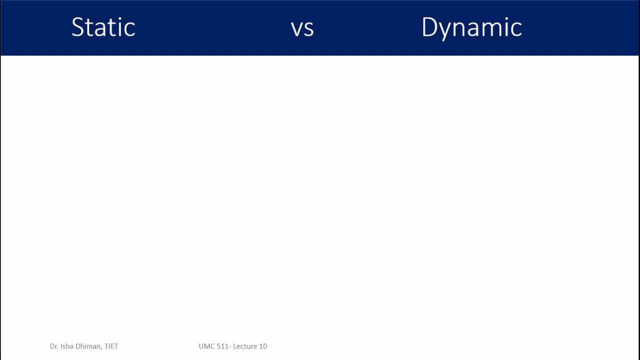 dynamic. this is very easy to understand. dynamic means anything is changing with respect to time, so everything is changing with respect to time all the time. you can say: everything precisely in this world is dynamic. nothing is constant, because the something is constant means it's dead, it's no more existing, it does not change, but anything which is continuously. 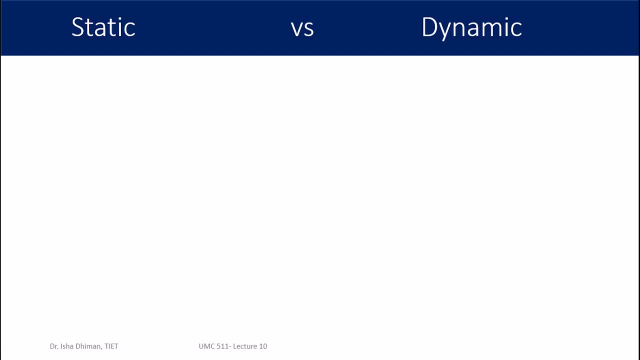 existing means. it is going a continuous change of state, so everything is dynamic. so now we want to understand the dynamics of particular process, so we model them with a dynamic version. otherwise we model them with a static version. so static means something when we have the models in which we have no. 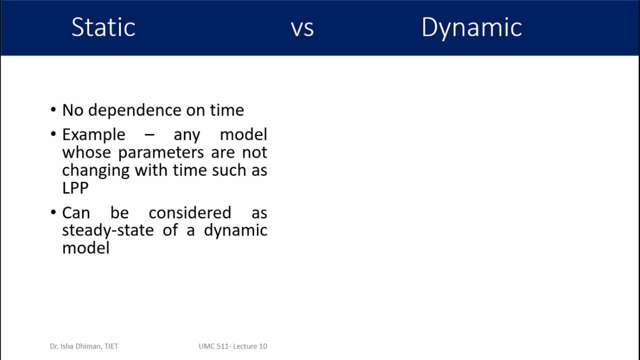 dependence on time. the things will not change with respect to time, for example, any model whose parameters are not changing with time. again, you can have the example of linear programming problem if somebody tells you that, okay, this much product you are manufacturing and this is the cost price, this is the. 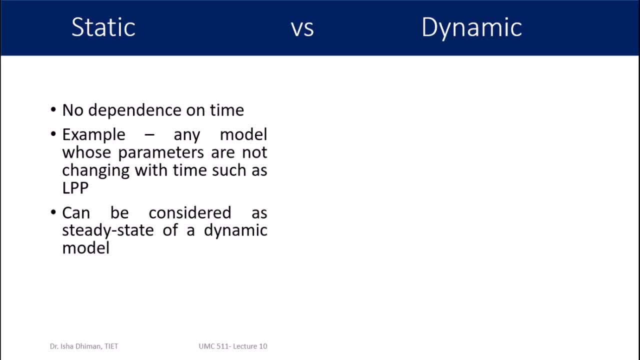 selling price. so you just assume that this cost price is constant, this selling price is constant. there is no dependency, there is no explicit dependency of the variables with respect to time. so those kind of models are static models in which time is not appearing explicitly. you can also say the static models are the steady state of a dynamic model. we 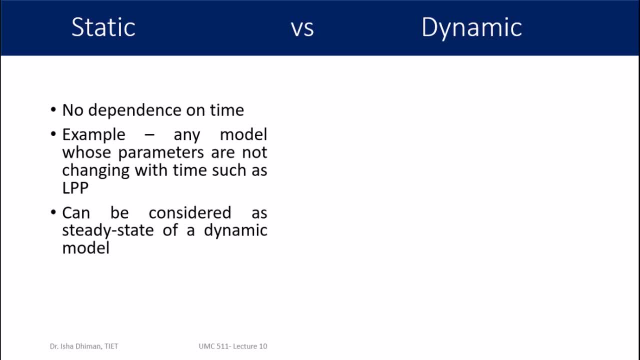 are already clear with the meaning of the term steady state. we have studied this in the population growth models. that steady state means that state when things stop changing with respect to time, d by dt becomes zero. so the static models can be studied under the particular case of dynamic models as 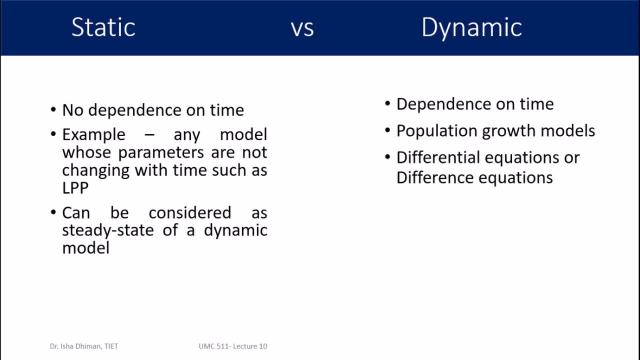 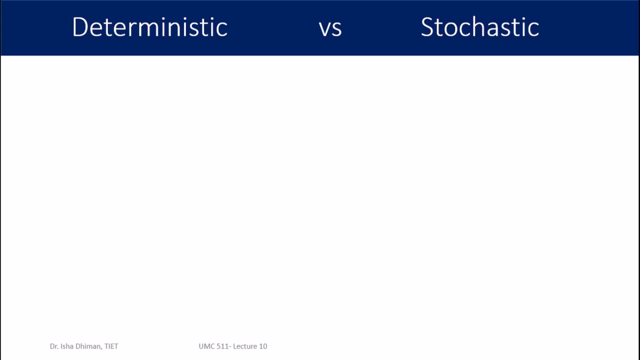 their steady states. so you can now understand that dynamic models have explicit dependence on time, for example, the population growth models, or the differential equations, or the difference equations. so many more models will be formulating which will be dynamic in nature. and now talking about another category, deterministic versus stochastic. this is 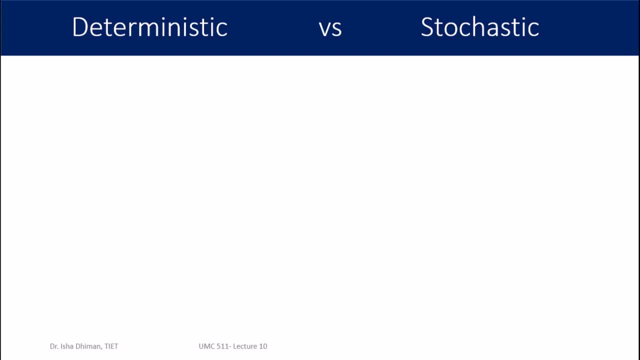 a new kind of category. you might not have been familiar with these words earlier, so let me put this into a detail. so deterministic means something which is certain. it is with full surety you can say that this is going to happen. so let me take the example of coin tossing. if you toss a coin then you are not sure. 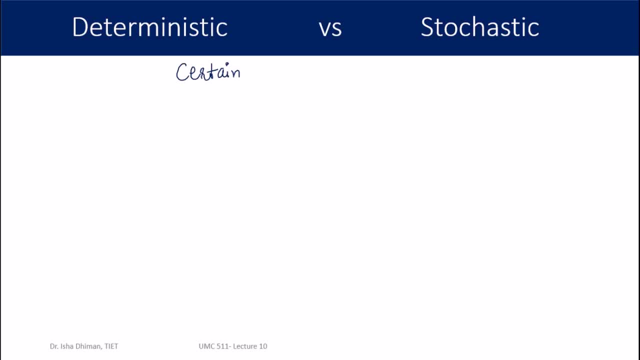 whether a head will appear or a tail will appear. so the occurrence of your output, or you can say the output of your event or the experiment, is not sure, with 100% surety, with 100% certainty. those kind of processes are the stochastic processes. so a coin tossing is a 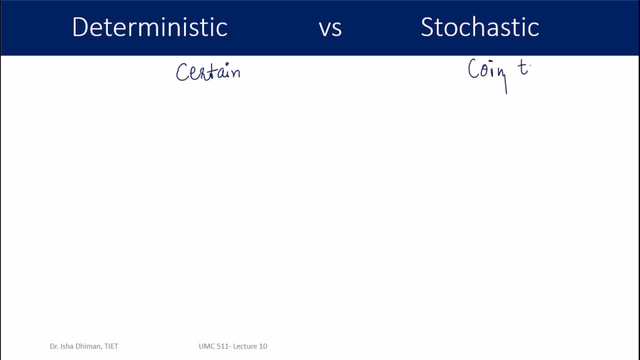 simple example of stochastic process, because the output is not 100%, certainly not sure whether head will appear or the tail will appear. on the other hand, in the deterministic kind of processes, the output is known to us that this is going to happen. for example, if i give you a 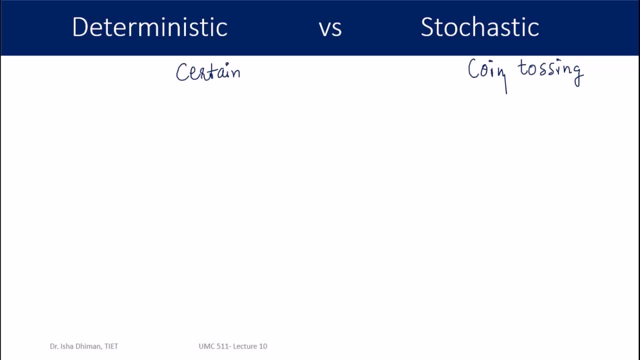 formula x square plus 2x plus 3. and then i tell you: put x equals to 1 in this, then every time you will apply the same formula and substitute the same value of x. you are going to get the same value. so those kind of models or those kind of processes are called deterministic. 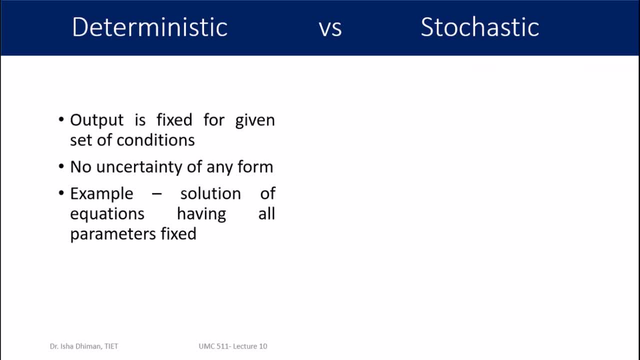 process. so in a deterministic model or process the output is fixed for given set of conditions, no uncertainty of any form. example solutions of equations having all parameters fixed. just now i gave you an example. say i ask you to find the roots of this equation. so if you find 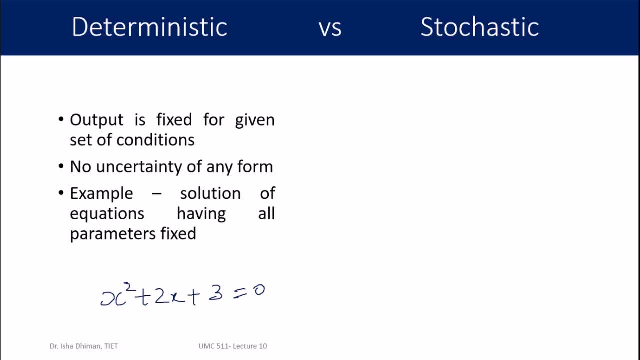 the roots today, you will get the some answer. if you will be finding the roots after some time, or maybe tomorrow, you will get the same answer every time. because if you find the roots today, you will get the same answer every time. because the output is fixed, it's not uncertain. however, this does not happen in stochastic. 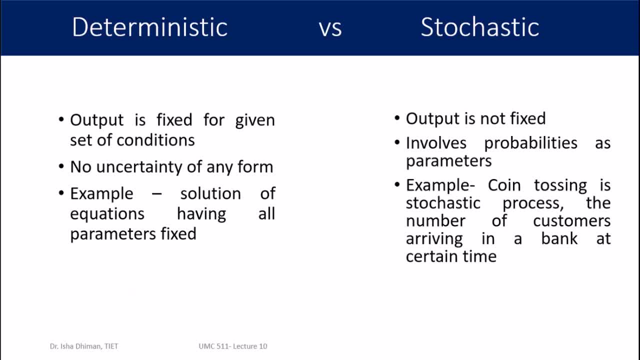 as i just gave you the example of coin tossing. in coin tossing, if you toss a coin today, maybe you will get a head. if you toss a coin tomorrow, keeping all other conditions same, then you may get a tail. so that's a stochastic process and to understand stochastic kind of processes we need 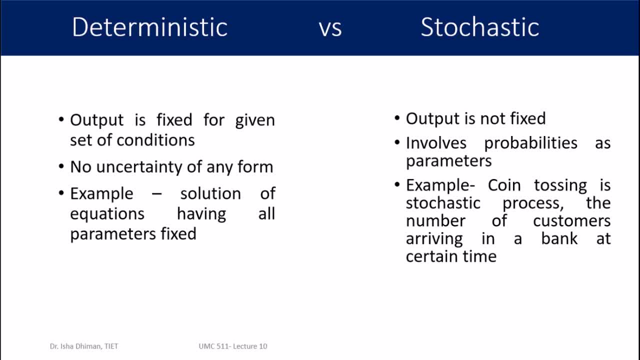 stochastic models. so that means our parameters need not be stochastic- deterministic. they should be in terms of the probabilities. so stochastic models are in general perceived to be better approximations of the real world phenomena- not always, but most of the time. our stochastic models are gaining more popularity with time as they are going to capture the 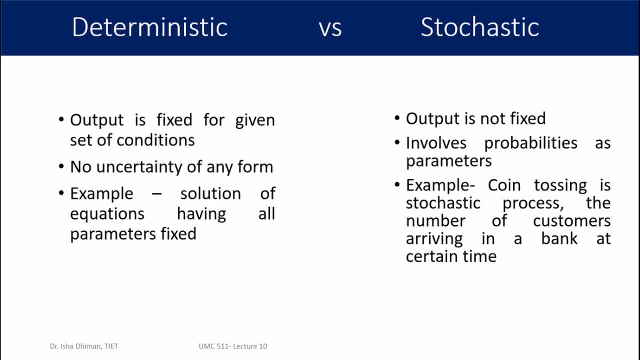 uncertainties of the real time processes more efficiently as compared to the deterministic versions. so we'll study about the stochastic processes in detail in the subsequent lectures, but right now this is just to understand the broad difference between deterministic and stochastic. so another example of stochastic is written over here. 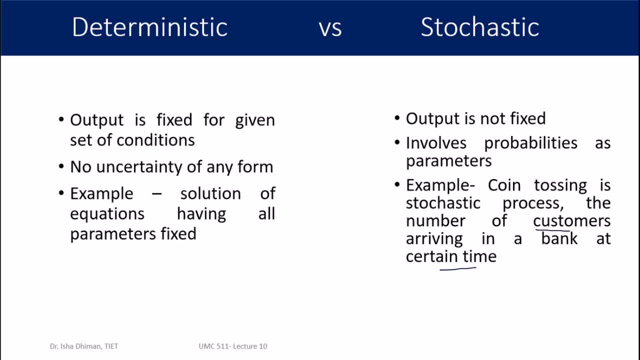 the number of customers arriving in a bank at a certain time is also a stochastic process. if you go to a bank and, at say, 3 pm, you count the number of customers arriving on one day, your data will be different. on another date the data will change, and similarly on third day. 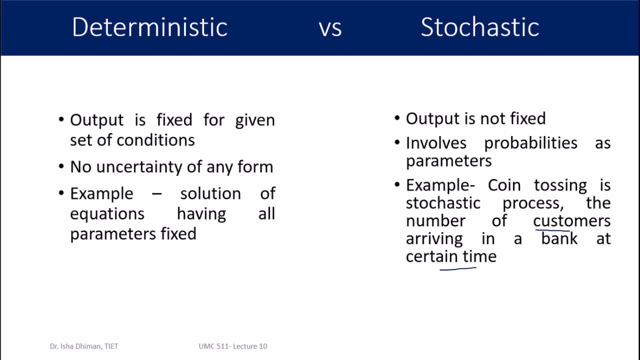 number is going to change and never, ever, you are going to be fixed about that. this day, this many customers will arrive. so that is also unpredictable output, or non-deterministic, or better called stochastic. so that's another category. and finally, i'm checking the last but not the least category. 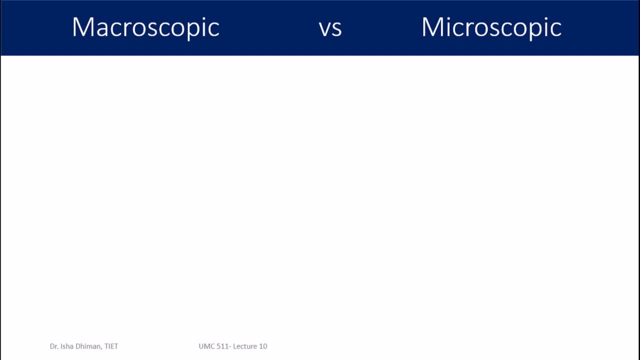 of mathematical models, which is macroscopic versus microscopic. so it's also literally clear from the meaning: macro means something needs to be studied at a macro or a large scale, and micro means studied at a micro scale. so it has to do with something with the level of detailing of the model we are. 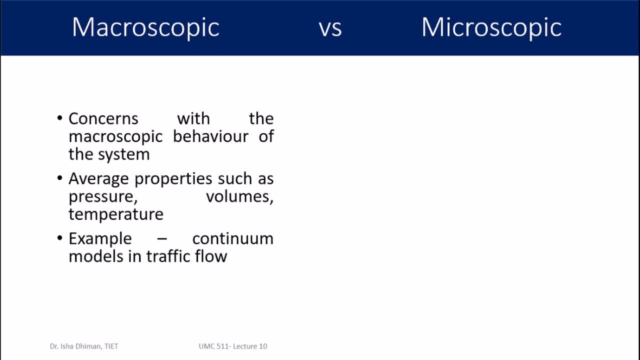 looking at. so macroscopic models concerns with the macroscopic behavior of the system. example: population as a whole. you are interested in how the population is going to increase. or you can say you are interested in how the population is going to increase, or you can say you are interested. 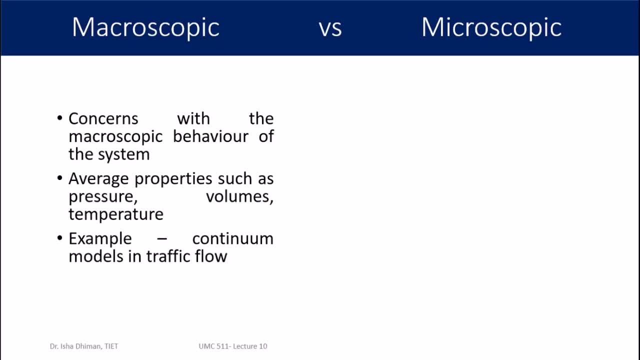 in looking at the average behavior of a population having large number of particles- human beings or whatever population you are considering- you are not interested in looking at their individual movements. for example, you have a large set of, say, molecules, so you are interested in the determining the average velocity of, the average speed of, or the average rate of diffusion of the gas as a whole. 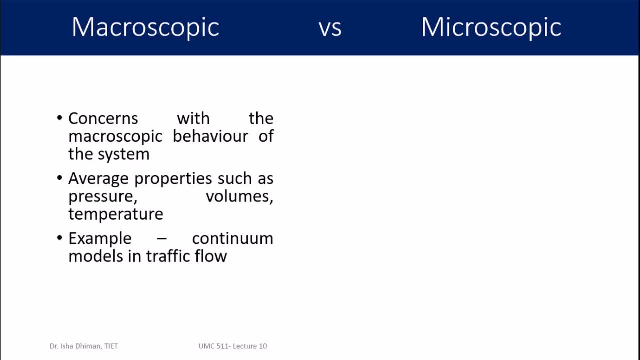 you are not interested in looking at the individual gas molecule and tracking its trajectory, so you are looking at the things from a macroscopic point of view, not from a detailed point of view. so here we are always interested in measuring the average property, such as pressure, volume and temperature. 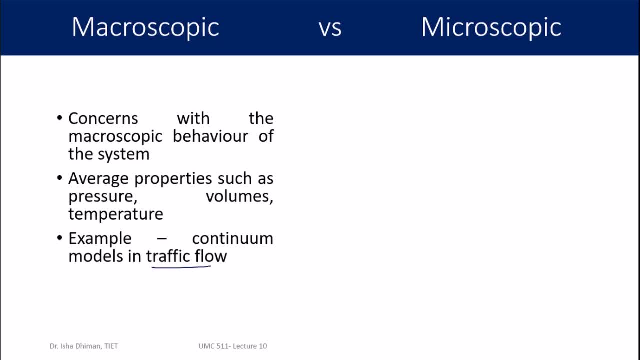 example, continuum models in traffic flow. so our next lecture is going to focus on this traffic flow, because this- actually this category- macroscopic versus microscopic- holds more sense in the modeling of traffic flow flow. so there, we'll be talking about these in more detail, but these are the